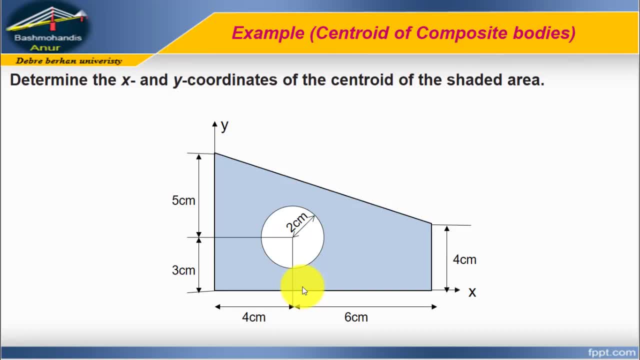 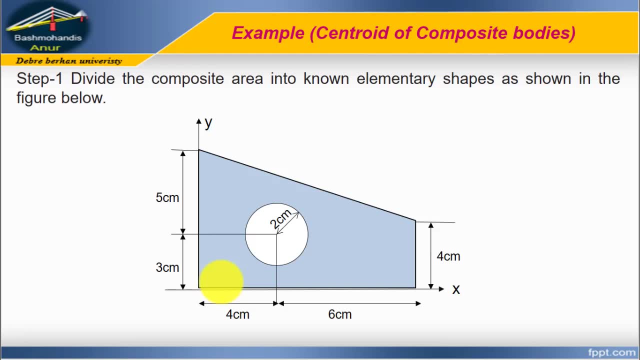 Let's find out the shape of the x function. Well, the first step is to divide the composite area into known elementary shapes, as shown. This is the general composite shape. I will show you a simpler shape later. First, let's see how to divide the composite shape into known and simple shapes. 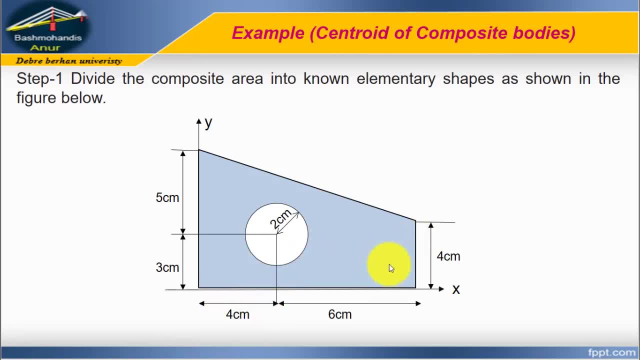 The first step is to divide the composite shape into 4 cm and 10 cm. Next, This is a triangle with a base of 3 cm and a base of 4 cm. This is a triangle with a base of 3 cm and a base of 4 cm. 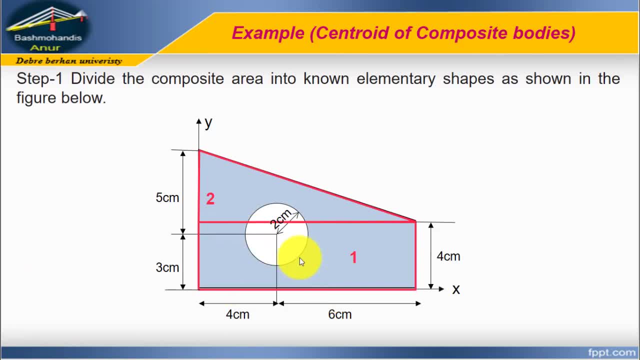 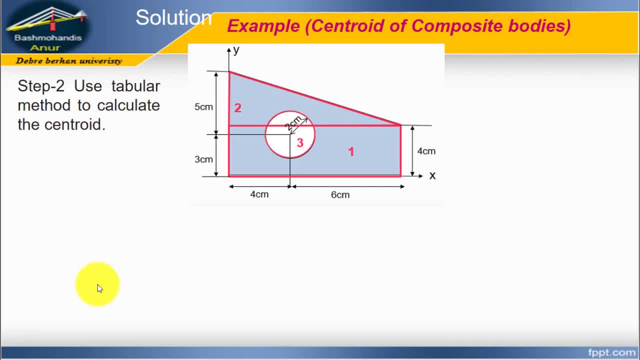 Because if you go to any engineering mechanics textbook you can find the centroid for each shape method. to calculate the centroid, Well, it's not a good data element table method, but it's the best option. by the way, It's a big, effective way You can. 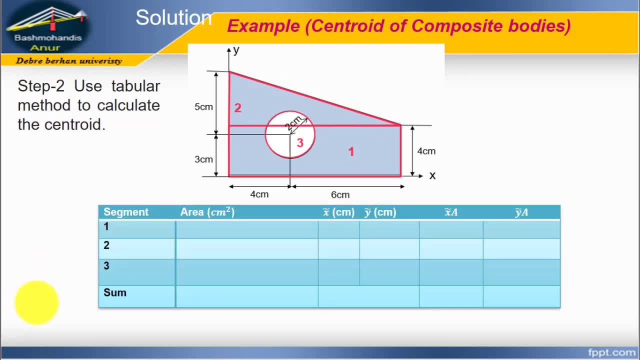 normally calculate matrix reality without using table. Well, table is very useful, by the way. It has column 1, segment, column 2, area to calculate matrix. column 3 is x coordinate, x tilde for each shapes. column 4 is y tilde, y coordinate for each. 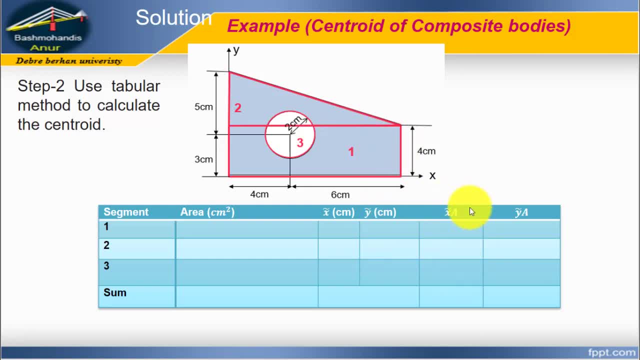 shapes. column 5 is x tilde times area. column 6 is y tilde times area. Okay, so let us start calculating of area for shape 1.. Okay, shape 1 is rectangle. Okay, rectangle area of any rectangle is base times height. Okay, base is 4. 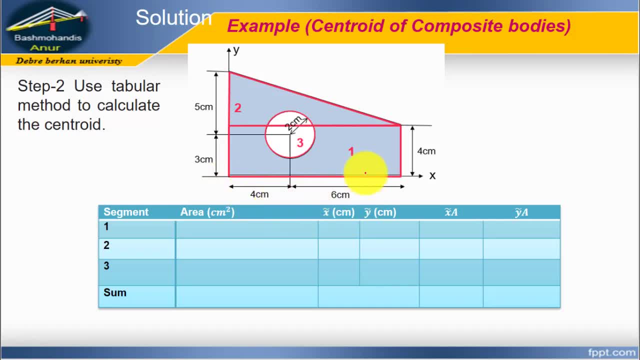 centimeter plus 1.. Okay, base is 4 centimeter plus 1.. Okay, base is 4 centimeter plus 1.. 6 centimeter, 10 centimeter. Okay, height demo: 4 centimeter, noise given Well. 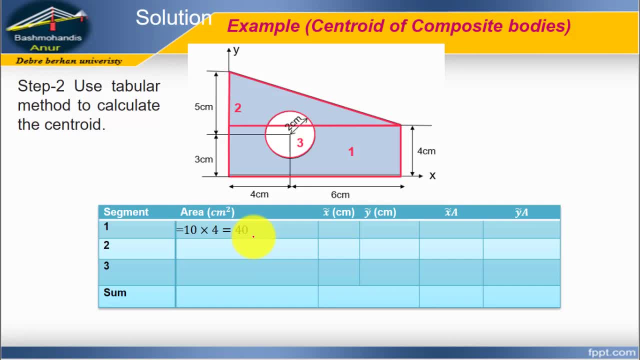 therefore, area for shape 1 equals to 10 times 4, which equals to 40 centimeter. Okay, next x tilde or x coordinate for shape 1.. Remember, guys, this is our origin. This is 0, 0.. x is 0, y is 0. So we have to calculate. 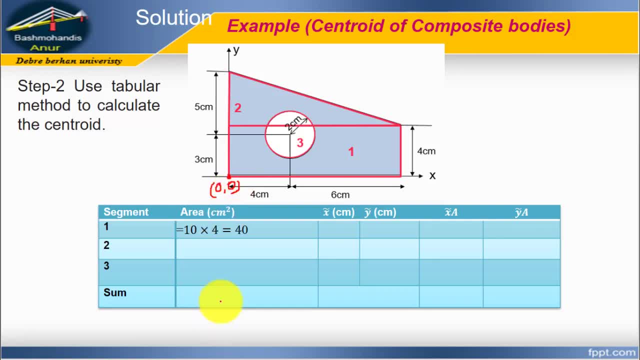 centroid of each shapes from this origin. Okay, how much distance should I go to get the center of each shape is from this origin, from this origin X and from this origin Y? well, for shape 1 it's rectangle, so from this origin I have to go B over 2 to get the center, X tilde or X coordinate for this. 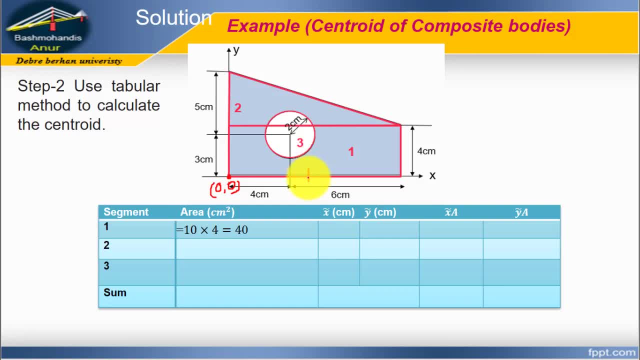 shape 1. yes, therefore, this is the test. this, approximately up to this one, is equals to B over 2, which equals to 5. well, we can write here 5 centimeter. well, what's Y tilde for shape 1? okay, from this origin we have to go H over 2. 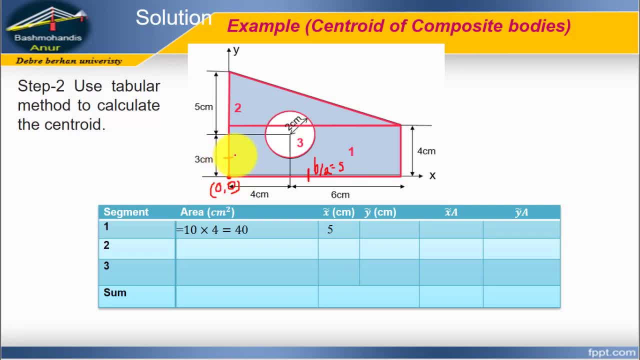 approximately up to this one. H over 2. okay, what is H? H is 4, therefore 4 by 2, which equals to 2, therefore, Ziga 2, that's available. well, this column, in this column, simply multiplying X, tilde with area, Y tilde with area, therefore X. 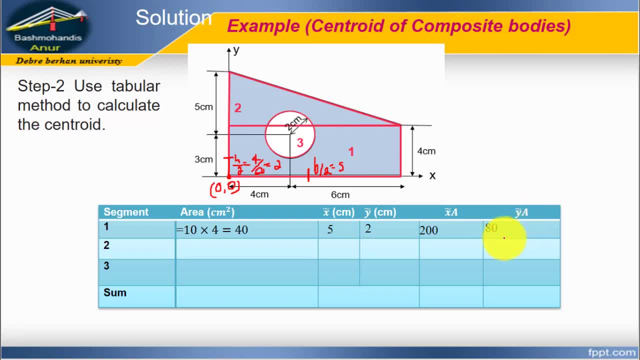 tilde times: area 200- imetal Y. tilde times: area 80- imetal. well, let's go next to shape 2. okay, therefore, area of shape 2 equals to you, because shape 2 is triangle. area of a triangle equals to one over 2 base times height. okay, therefore, the base for shape. 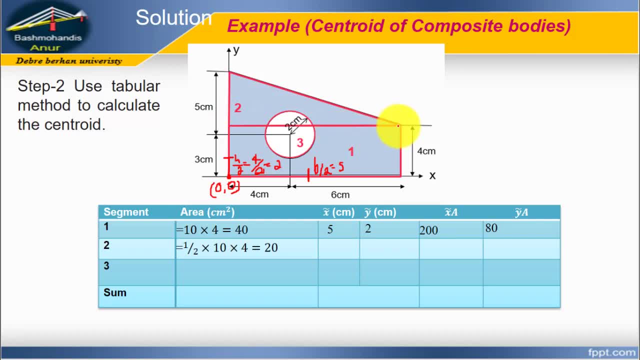 2 is 4 meter plus 6 meter equals to 10 centimeter and hate or H for shape. 2 is 4 centimeter. don't use 5. 5 is from the center of the circle. okay, it's not rainfall. x yani hı zgan. 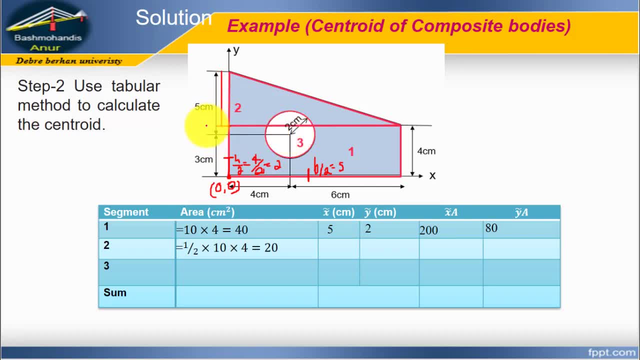 not the head of chef. therefore, hey, lauosa y숨 began × zero Lucka, I know it's not the head of a chef. therefore, shape 2, therefore, shape 2 is equal to 4 centimeter. okay, and then we can write this as 3 and this as 4, so this is from 4 minus 3. 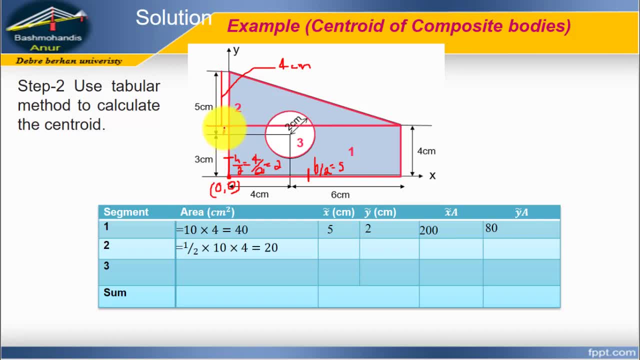 this distance is 1. okay, once we know that this is 1 quarter, total is 5, no k: 5 and 1. subtract 1 from 5 is equal to 4 centimeter. okay, therefore, height equals to 4 centimeter. therefore, 1 over 2 base times 8 equals to 20. 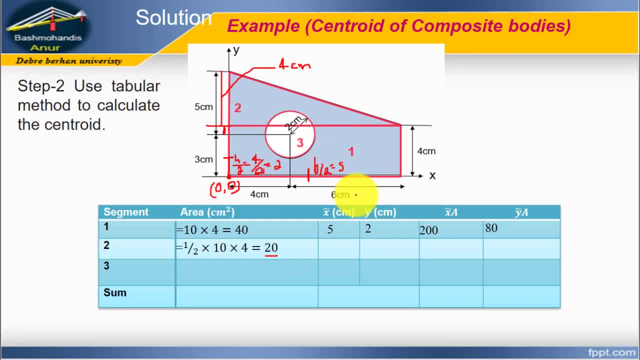 centimeters square area for shape 2. okay, what is X coordinate for shape 2? well, remember, this is our origin. okay, shape 2 is triangle and its origin for shape 2 is this one. okay, however, from the XY coordinate is from here. therefore, we have to calculate the centroid from this point up to the 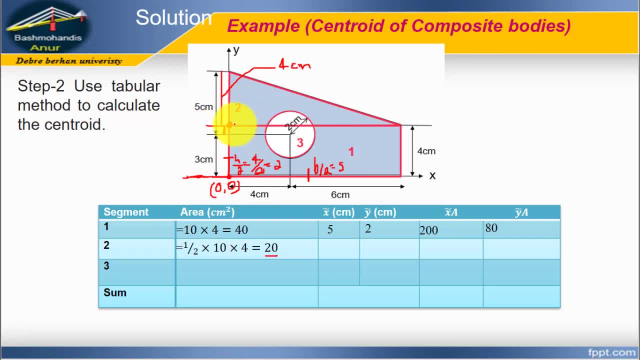 triangle in X and Y direction. okay, therefore, from this, from its origin, from this corner, we have to go B over Street gate centroid interval, So that we have to have 3 centers for this point in this general operation. okay, therefore, from this, from its origin, from this corner, we have to go B over 3 to get centroid in this. 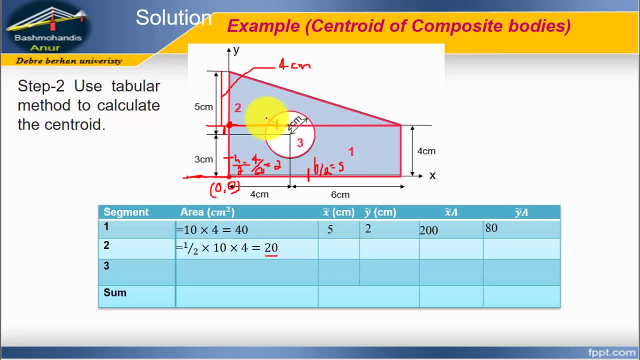 the x-direction. okay, therefore, yes, in terminal, a bit: B over 3, B 10, no. therefore, this equals to 10 over 3. well, what about 10 over 3 gamma's of a level? what about? why, kawaii domo, Kazuma, Minnesota level? we have to go from here. 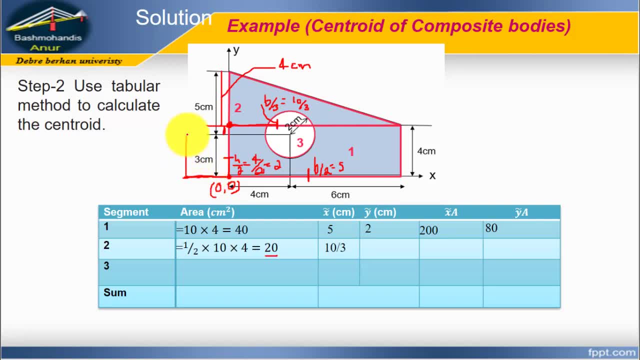 therefore, up to first, from this up to this, yeah, are at centimeter for centimeter. what about from this origin, from its origin, not from the XY from its origin, the triangle. up to this, we have to go B over 3 from the 90 degree corner. 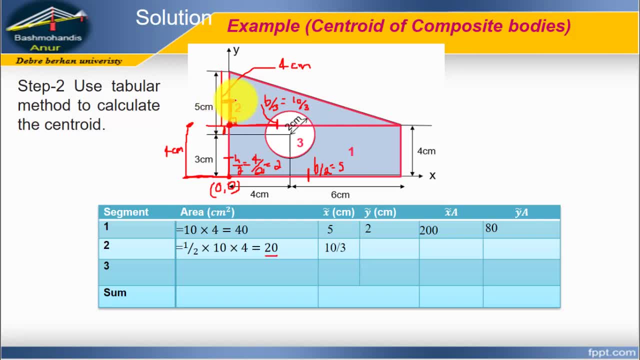 okay, sorry. H over 3. a. therefore this equal to H over 3 over 3, which equals to 4 over 3. okay, therefore, 4 over 3 plus 4 centimeter equals to 16 over 3 centimeter. Matt Alma, let's not okay, okay. X till the times area. 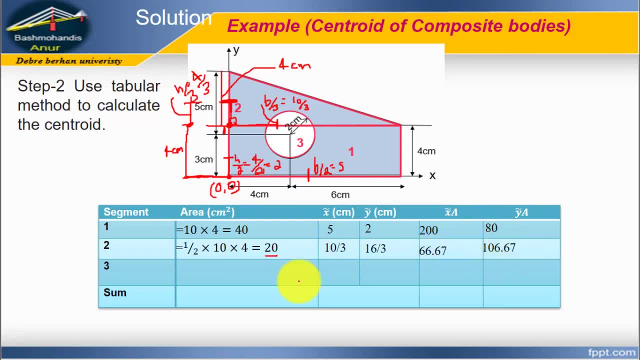 now wait till the times area. simply my buzzard. no, yeah, Matt Alma, let's not. okay, what's left? shape 3: okay, shape 3. what's left? shape 3- okay, shape 3 area equals to pi R square for any circular. area equals to pi R square for any circular. 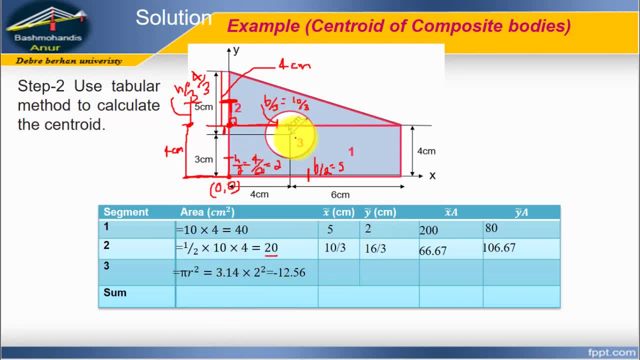 area equals to pi R square for any circular section. okay, therefore, radius is section. okay, therefore, radius is section. okay, therefore, radius is given to centimeter. therefore, remember, here we given to centimeter. therefore, remember here we given to centimeter. therefore, remember, here we have to put negative sign. why 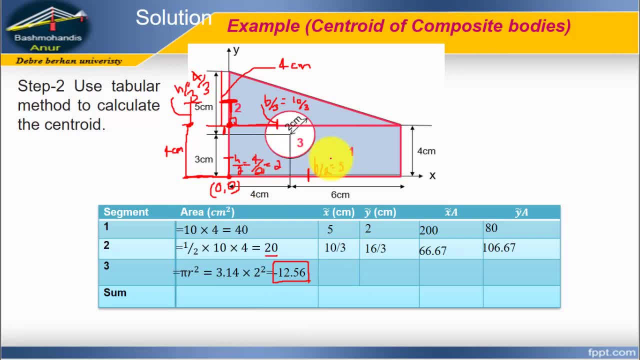 have to put negative sign. why have to put negative sign? why? this is because we are calculating. this is because we are calculating. this is because we are calculating centroid for the shaded area, however, the centroid for the shaded area, however. the centroid for the shaded area, however, the circular is not shaded, it is hollow. 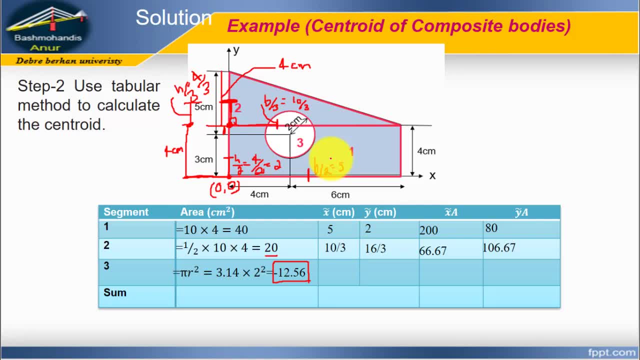 circular is not shaded, it is hollow. circular is not shaded, it is hollow circular section. therefore, the area must circular section. therefore, the area must circular section. therefore, the area must be subtracted because when we calculating be subtracted, because when we calculating area of the shape 1, we consider it as a solid and shape 2, we consider it as.